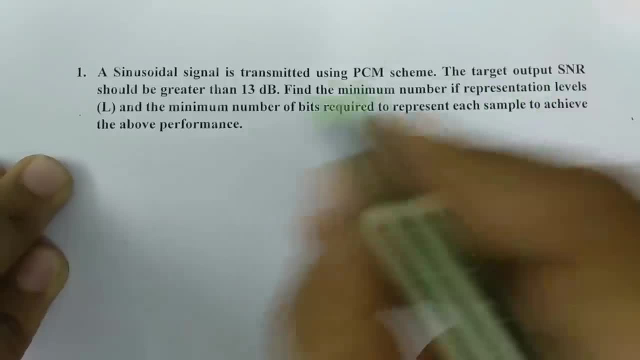 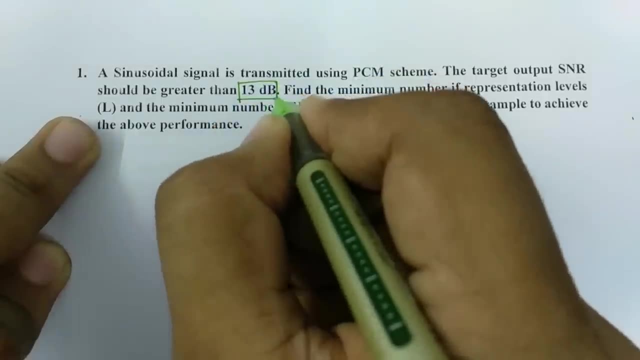 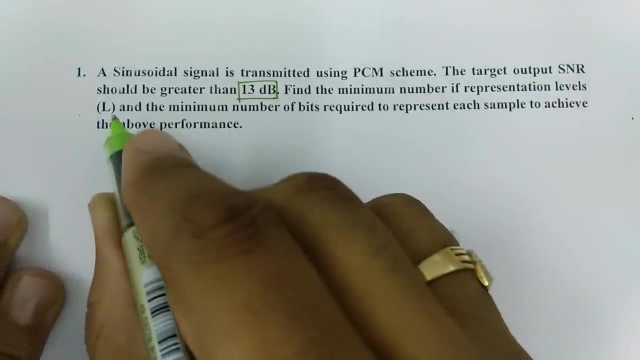 input is sinusoidal, The target output SNR, should be greater than 13 dB. So here, SNR that should be greater than 13 dB. Find the minimum number if represent level L, and the minimum number of bits required to represent each sample to achieve above performance. 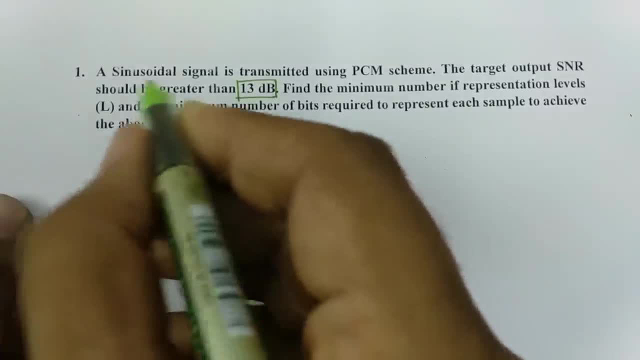 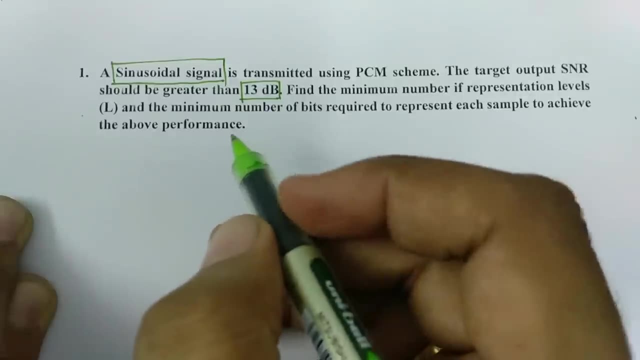 So here, one thing that is so essential, which is signal, is sinusoidal. Now see, if signal is sinusoidal, then calculation will be very easier, and for that, all the formulas that we have derived and we will be able to solve this problem. So let us begin this session. 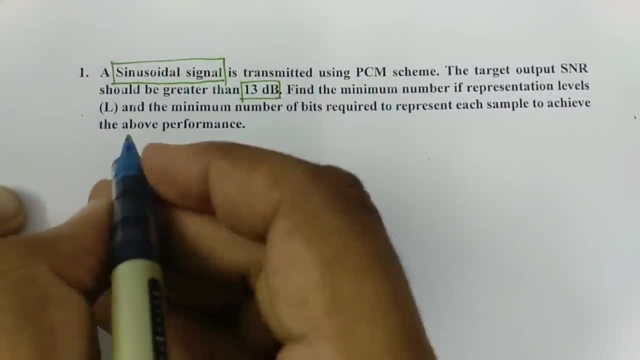 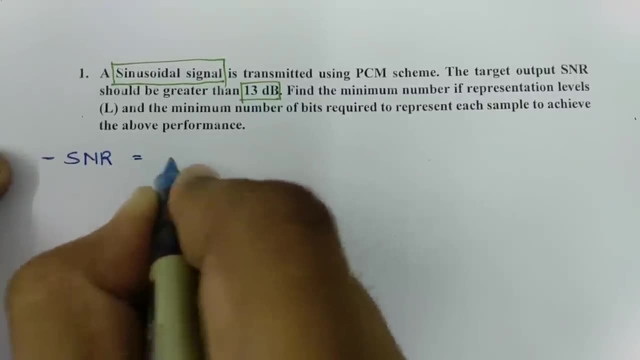 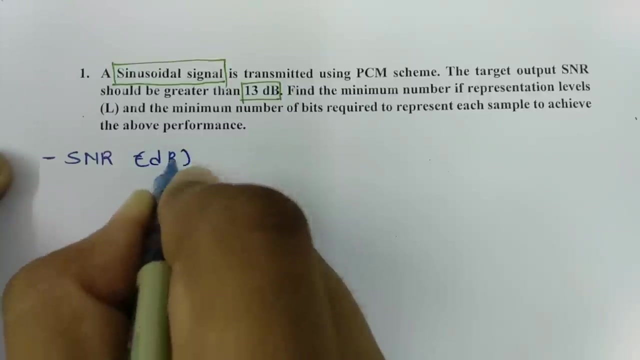 And based on those formulas we will be solving this problem. So here, as we have derived SNR, so SNR that will be. that is actually 13 dB that is already given in terms of dB, SNR in terms of dB that is given by 13, and we know the basic formula which we have derived, that is: 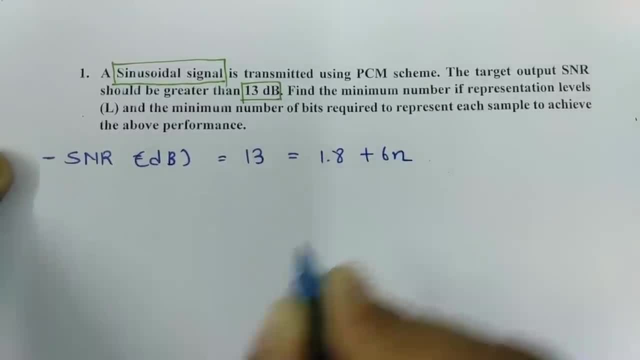 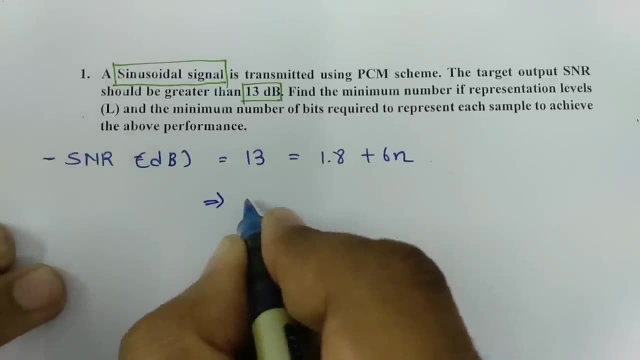 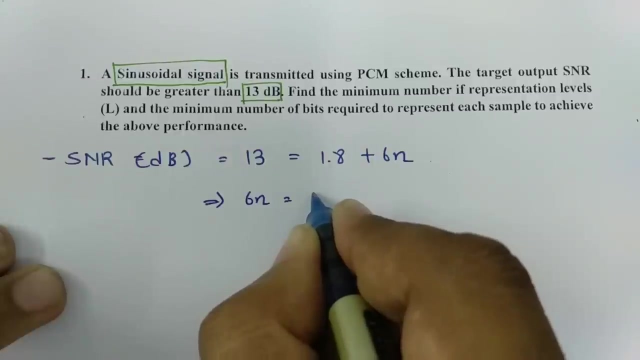 1.8 plus 6 n, where n is number of bit which is required. So that is today. we don't tell you again what is the blessing of counting n, But initially we will run some easy by gjuba byhmm. So in this video we'll 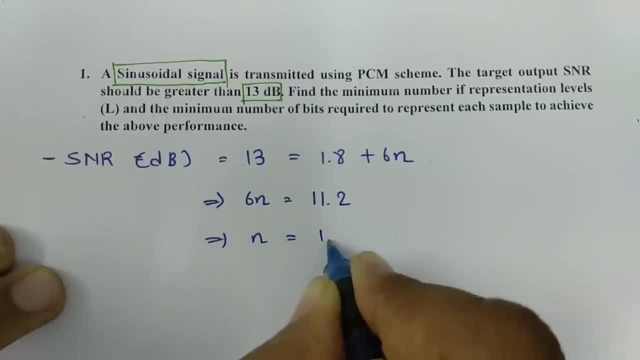 take deterministic terms, be using write most will be a total of eight. so to have a set same number of n will be equal to i, 2 to j times 16 by 6 by n pants holds to 5. That will be equal to 6 N minus 8. that represent a sample. So based on that we can say 6 n, that is 13-1.8.. That is 11.2. and if you further calculate the number of bits then that will be one point 86.. Now we need to take number of bits in. 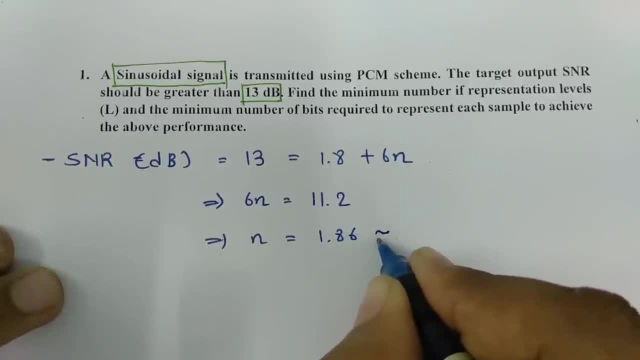 terms of integer. the reason is you cannot represent number of bit, So we will seed star team. Number of bits will be 1233 times anyway. Now, power of the numbers of on the Predator constant is. So we will be taking integer value. that is what 2.. 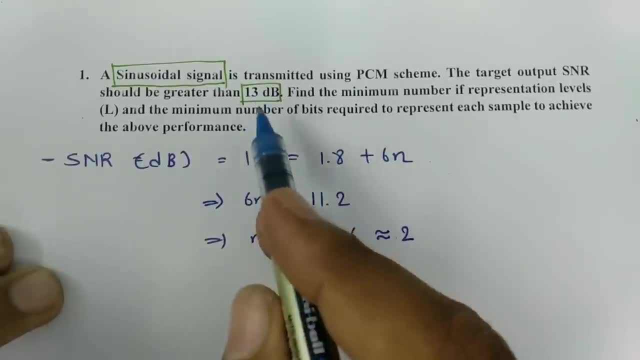 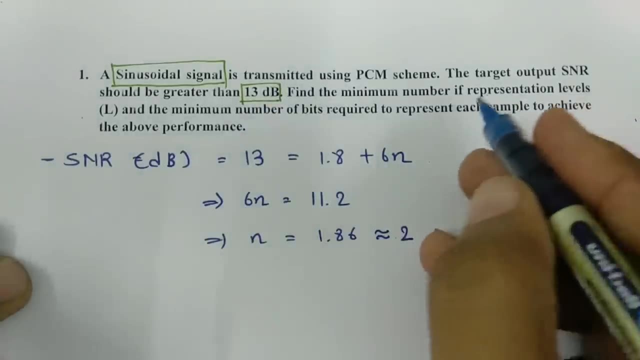 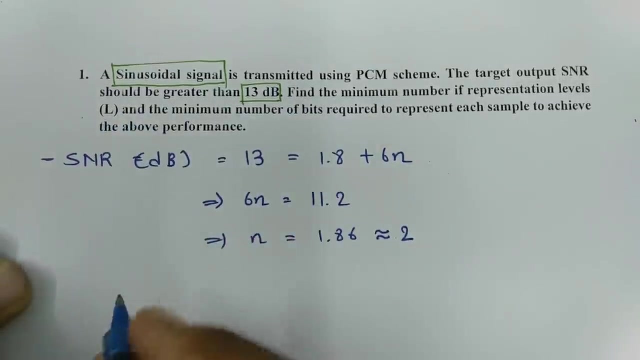 So 2 bits are required to represent that sample, as per SNR should be greater than 13 dB. Now, number of bits that we have calculated. Now we will be calculating number of samples represented by that bit. So number of samples that we can calculate by 2 to the power n, where n is 2.. 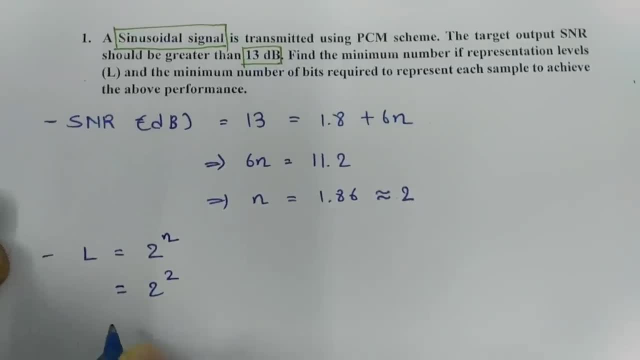 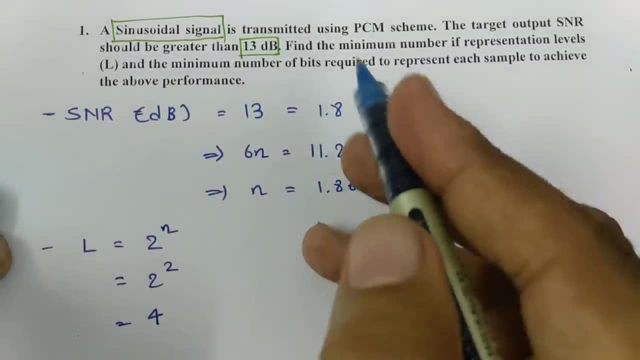 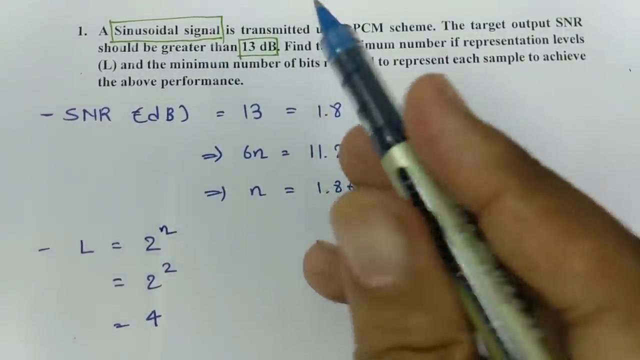 So if you place that value 2 to the power 2.. So we will be getting, this is 4 samples, So total 4 samples that we can have to represent any individual signal transmitted as per the sinusoidal signal. So this is what we can represent by this system. 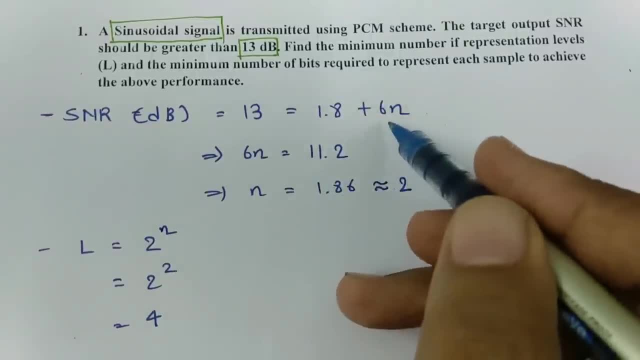 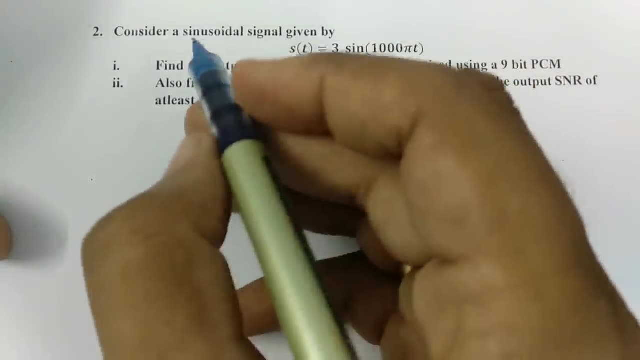 So number of samples as well as number of minimum bits that we have calculated in this question, Now we will be calculating next question Here again. here consider: Consider: a sinusoidal signal given by S of t is equals to 3 into sin of 1000 pi t. 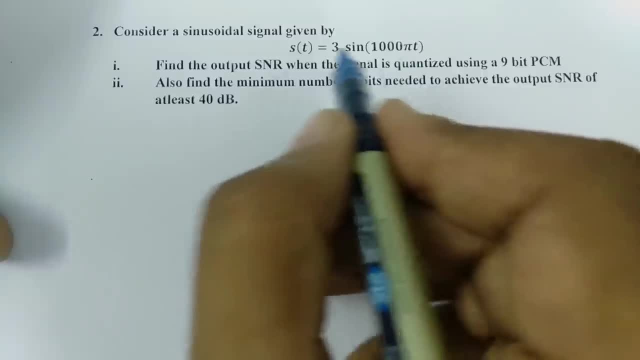 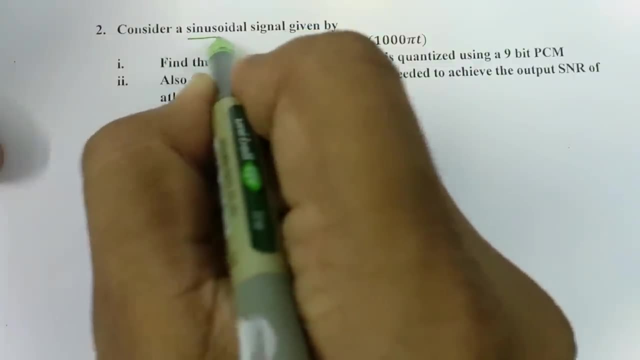 So signal is given by 3 sin of 1000 pi t. Now here again one thing that is very clear to all: Signal is sinusoidal. Input signal is sinusoidal, So this is so essential to understand: Input signal is sinusoidal and that is what this signal 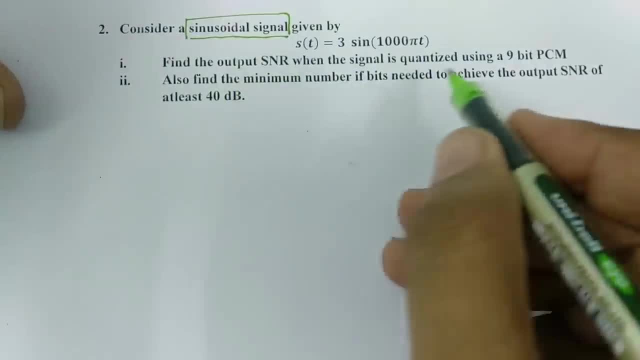 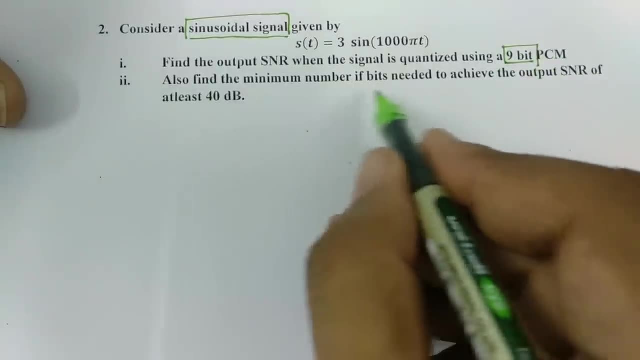 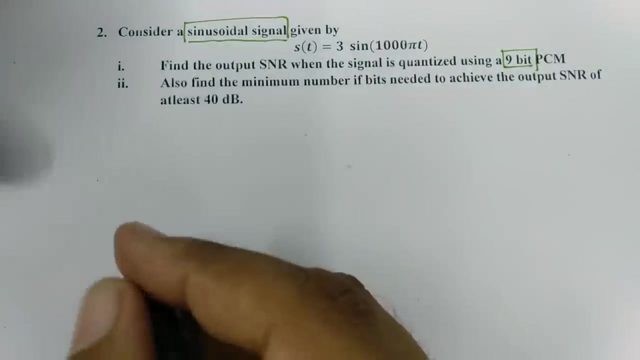 Now question is: calculate SNR when the signal quantized by 9.. So we can find the minimum bit and also find the number, minimum number of bits needed to achieve output SNR of at least 40 dB. So if PCM is described by sinusoidal signal, in that case we have fixed formula. 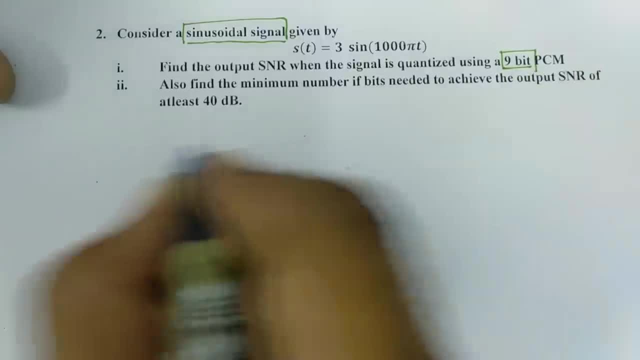 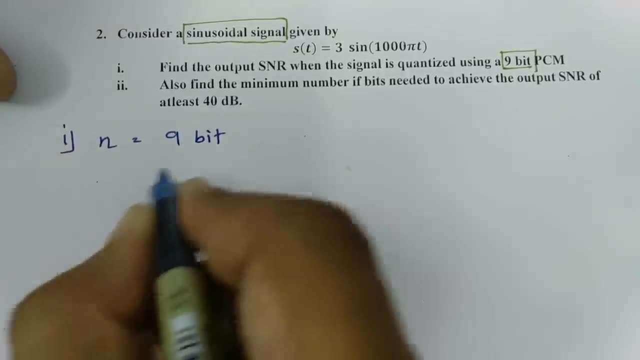 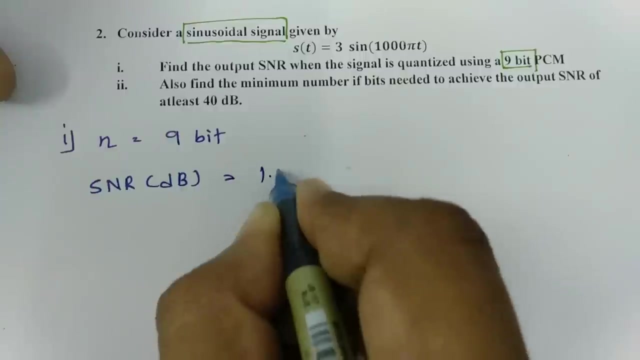 And for first question we have 9 bits. So for first calculation n is equals to 9 bit. So now SNR that we can Calculate as per in terms of dB. we can calculate this by this formula: 1.8 plus 6 n. 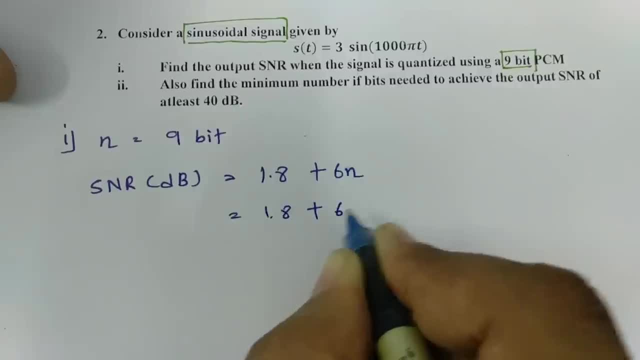 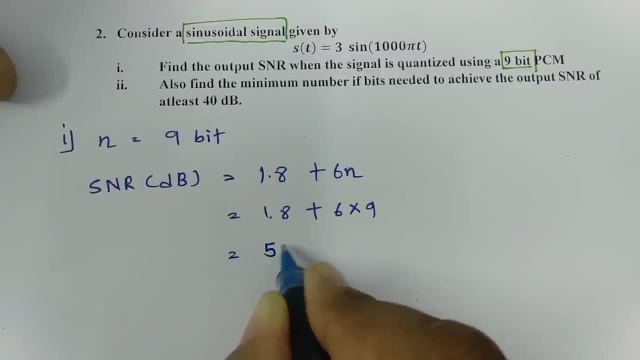 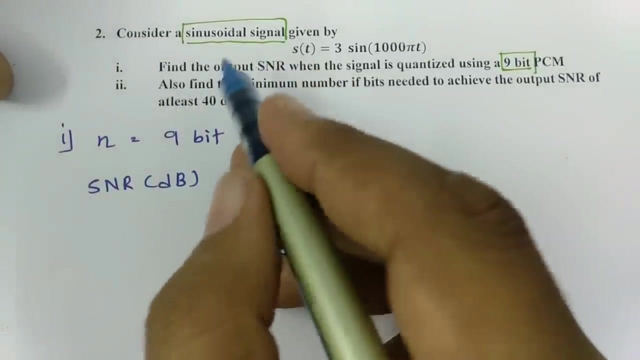 And if you place values 1.8 plus 6 into 9.. So 9 into 6, 54 plus 1.8, that is 54 plus 1.8, that is 55.8 dB. So this will be the SNR. for first case given input signal is this: 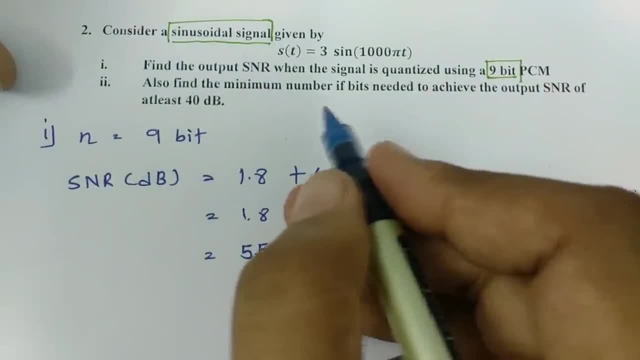 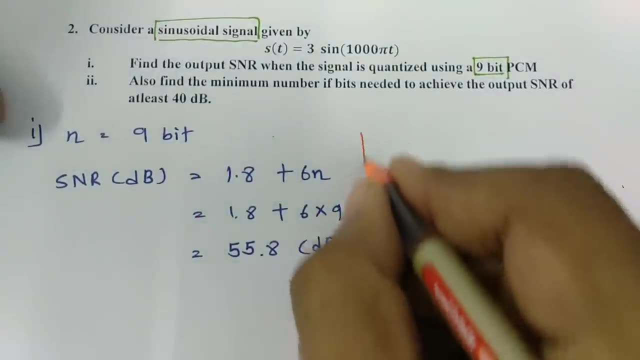 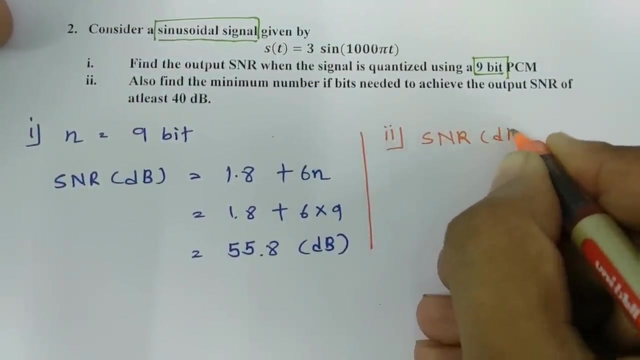 Now second question is also find minimum number of Bits needed to achieve output: SNR of 40 dB. So in second question, in second question, we have SNR that is given in terms of dB. it is given, So it is 40 dB. 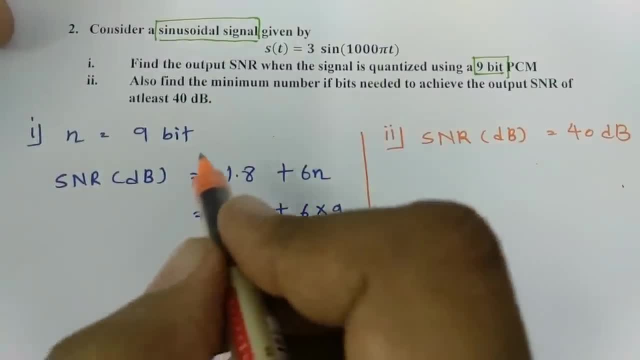 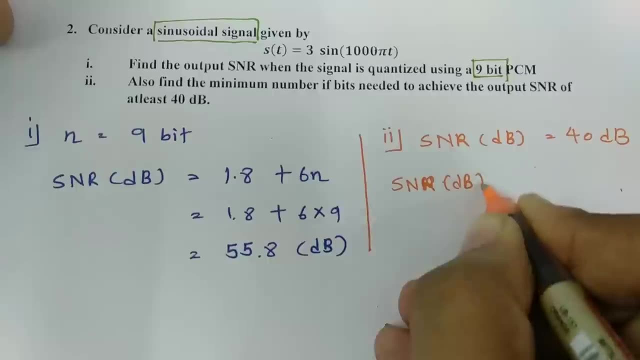 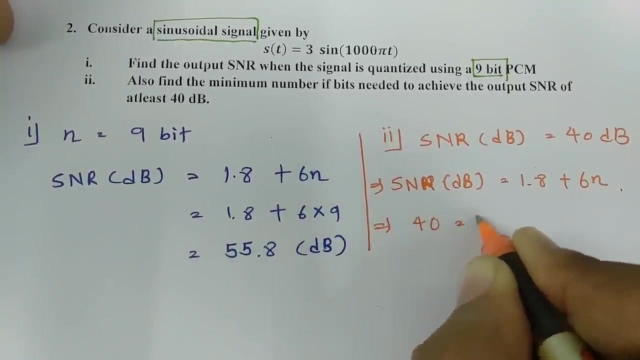 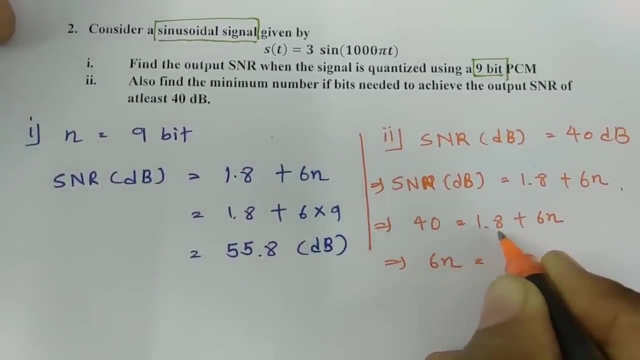 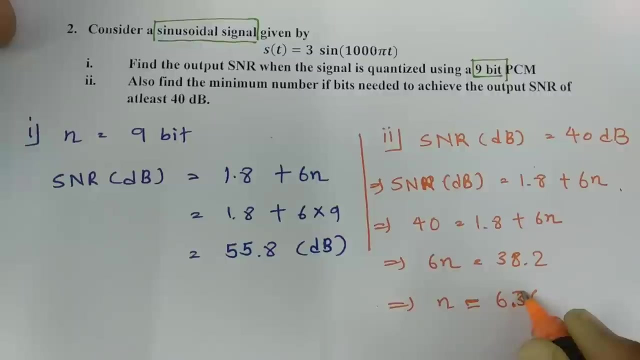 So we are ready to calculate minimum number of bits required to represent that. So we can calculate that by SNR. in terms of dB, That is 1.8 plus 6 n, and if you place values, 40 is equals to 1.8 plus 6 n, so that will be 6. n is equals to 40 minus 1.8, that will be 38.2, and if you do this division so you will be getting n is equals to 6.36. now see here. 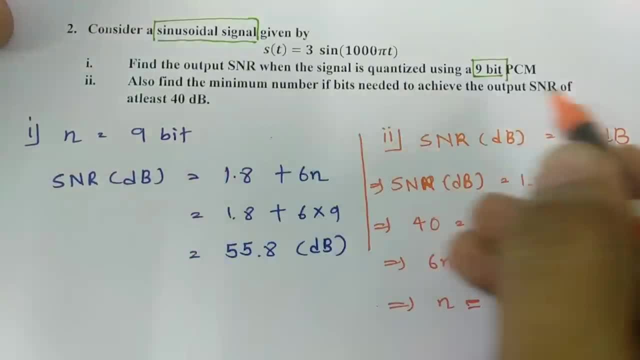 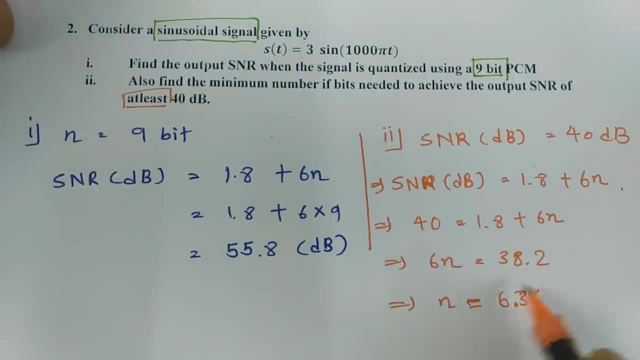 So this is what: n is equals to 6.36. but here we need to achieve SNR. at least 40 means we need to take n is equals to greater than this. So if you take round off over here, then you will have to take n is equals to 7 bits. 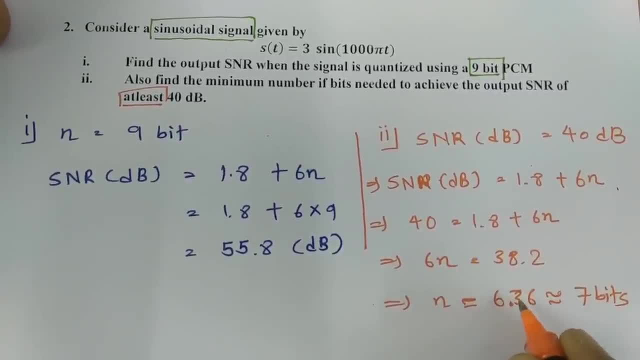 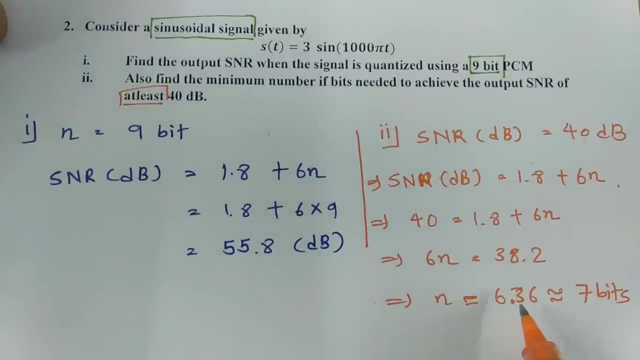 You cannot take lower than this. So you will have to have round off at greater than this, at fractional value, And that will result into 7 bits. If it is not at least 40 dB, in that case one can take 6 bits. but here at least this means accuracy will be more, so SNR will be greater than 40 dB if you take 7.. 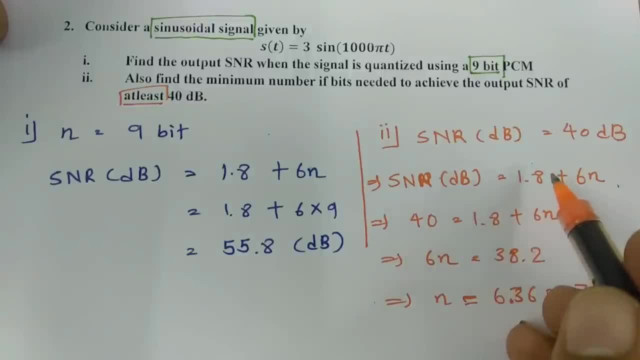 So if you take 7, it will be 6 into 7, that is, 42 plus 1.8, it will be 43.8.. But if you take 6, in that case SNR will be 6 into 6, that will be 36.8.. 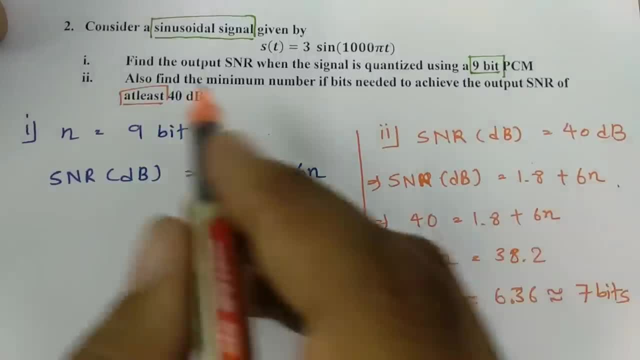 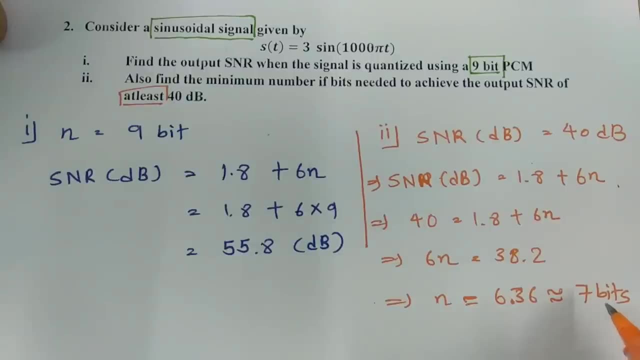 So if you take 6 plus 1.8 it will be 37.8, means it cannot achieve at least 40 dB. So when you do round off, remember this- you will be doing round off at greater value than the value which you calculate and do round off. 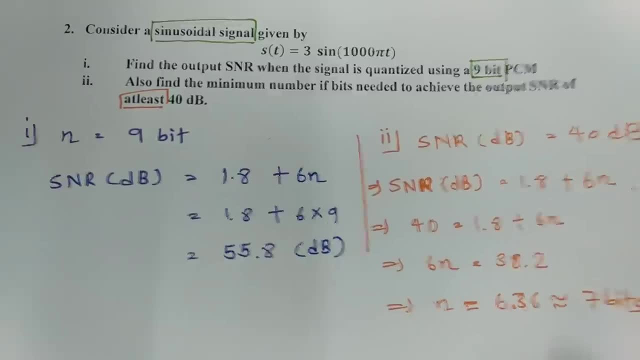 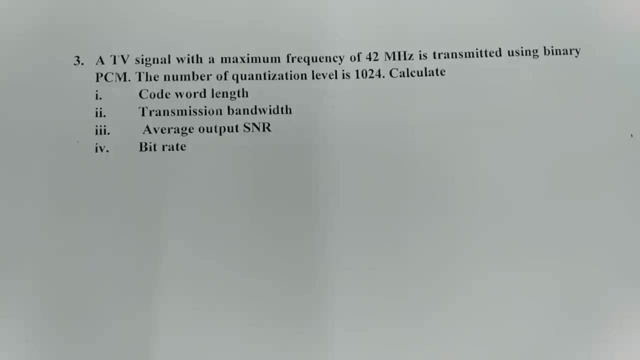 So this is what one should keep in their mind when they solve these examples. Now let us move on to another example, So that will be giving you little more idea how to solve this kind of problems. You just see this problem first. 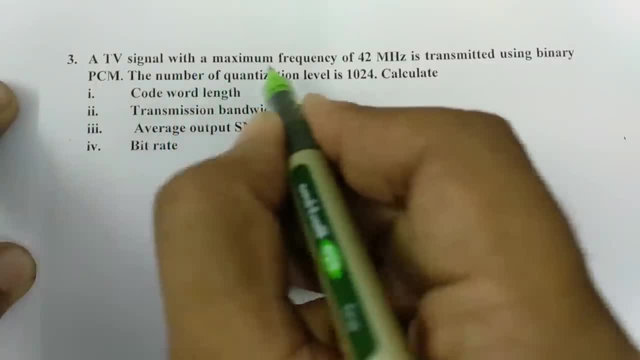 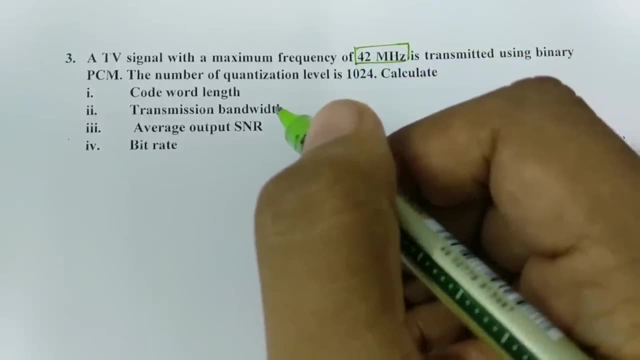 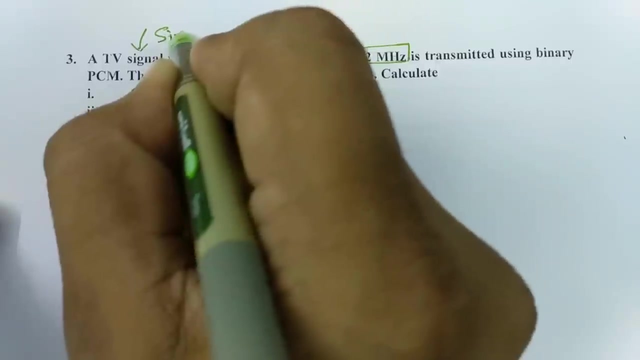 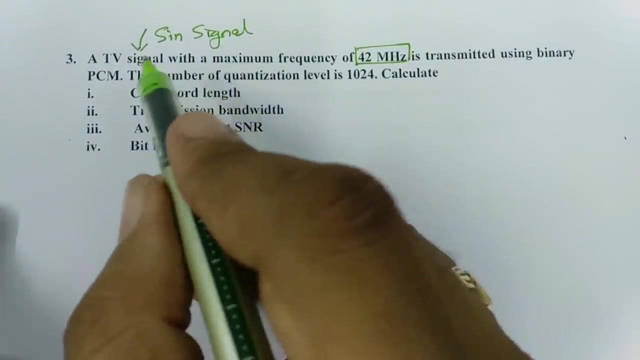 Now see in this problem a TV signal with a maximum frequency 42 MHz. Now see one thing that one should understand here: this is what TV signal and TV signal that is sinusoidal sign signal, TV signal, that is sign signal. So here even we will be using same formulas as we have derived it. 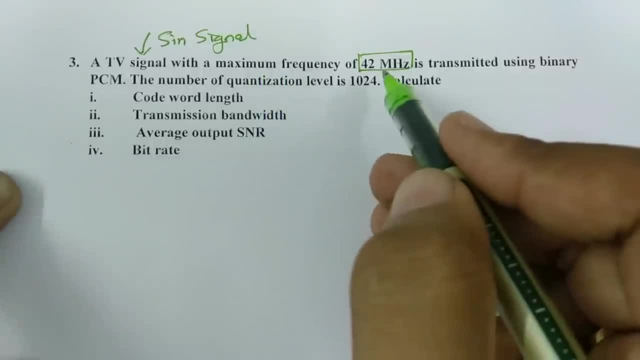 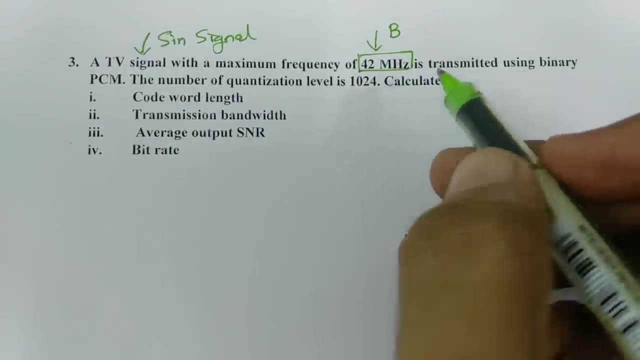 So for TV signal it is sign signal and that is having maximum frequency. 42 MHz means bandwidth of signal that is given 42 MHz And that is transmitted by using binary PCM. The number of quantized level is even given, that is 1024.. 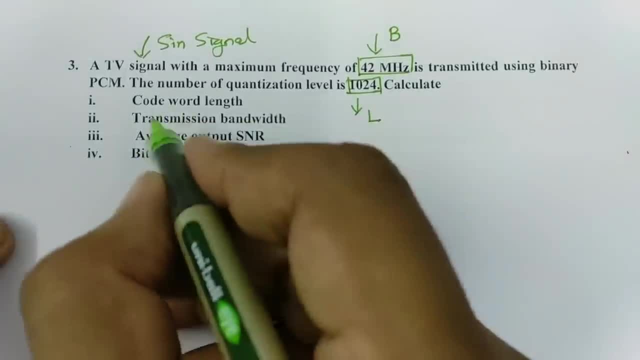 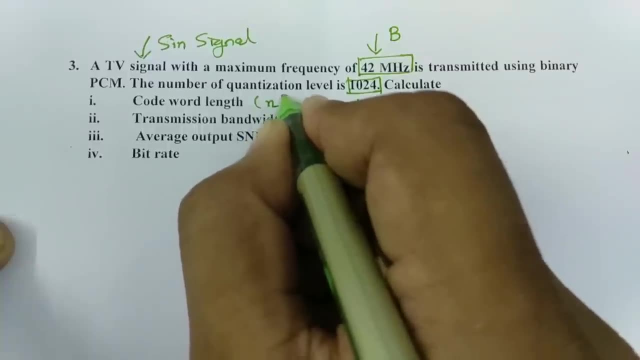 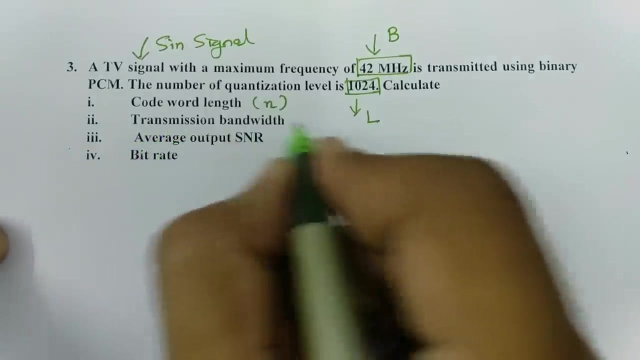 So L is given, that is 1024. We are delivered to calculate code word length means we are delivered to calculate number of bits per sample. means N, Number of bits per sample, that is what code word length. Then we are delivered to calculate transmission bandwidth, then average output, SNR, and at last we will be calculating bit rate. 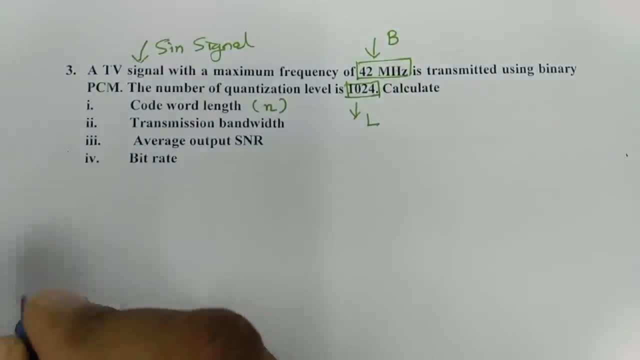 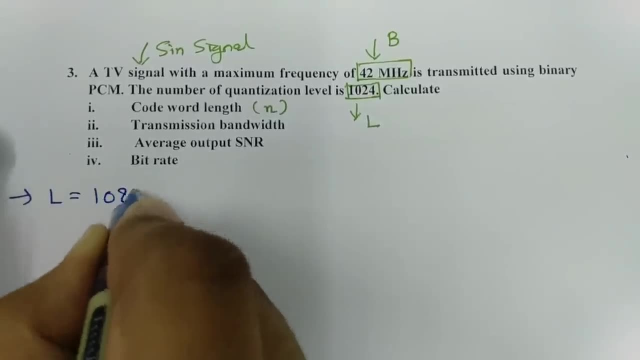 So let us solve this step by step. So see here: L is given, So L is equals to 1024.. And to calculate N code word length, we already know L is what 2 to the power N, So L is equals to 1024. 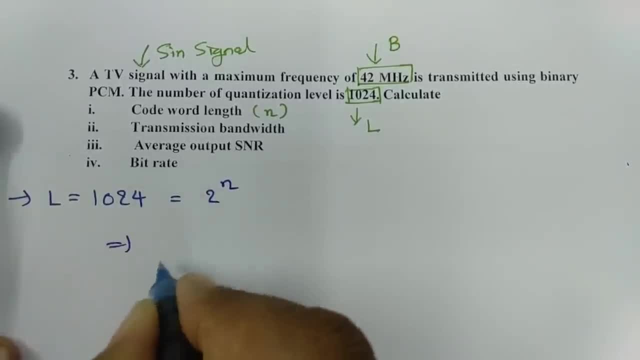 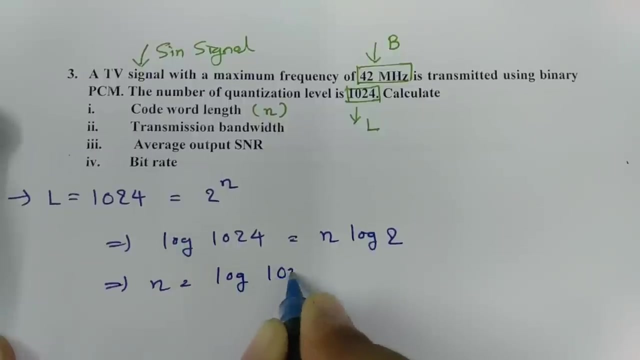 So to calculate this we need to do log at both of the side. So log of 1024, that is equals to N times of log of 2.. So if you do this calculation you will be getting. N is equals to log of 1024 divided by log of 2.. 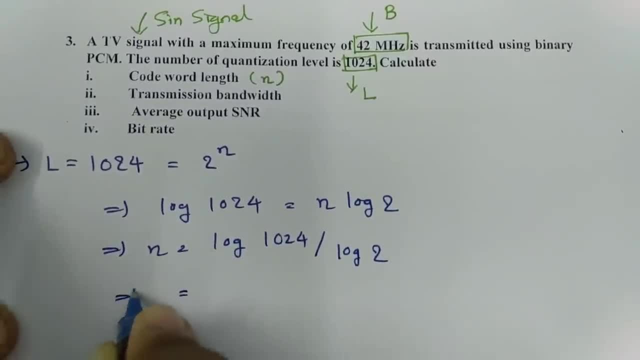 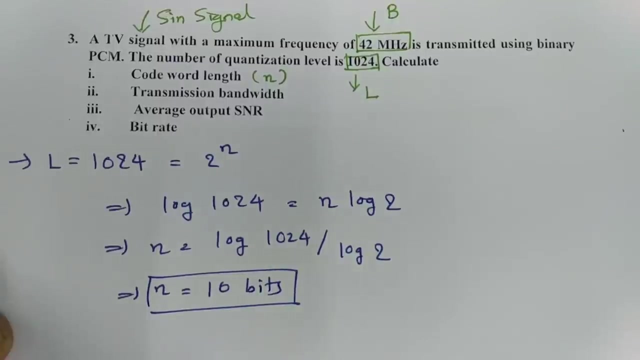 And that calculation will result into 10.. You just do it in calculator. you will be getting. it will be 10 bits. So code word length first answer: that is 10 bits. Now we are delivered. to calculate transmission bandwidth: Now see first of all what is transmission bandwidth. 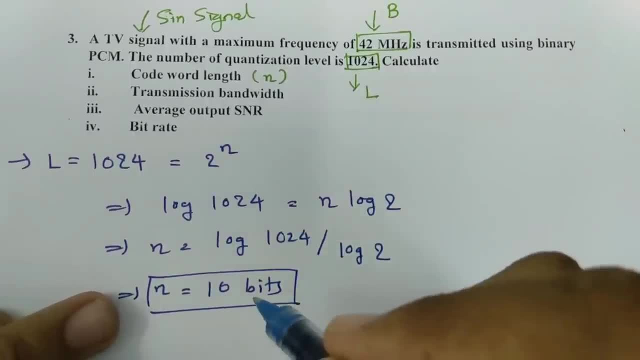 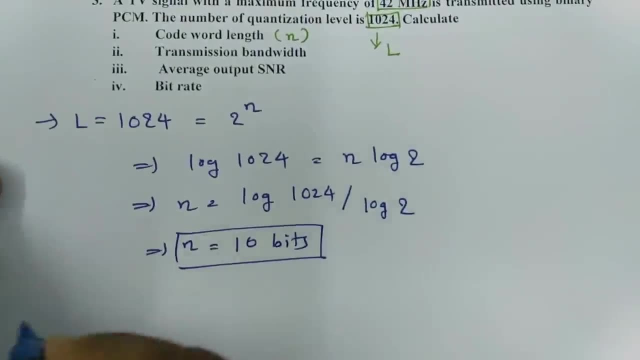 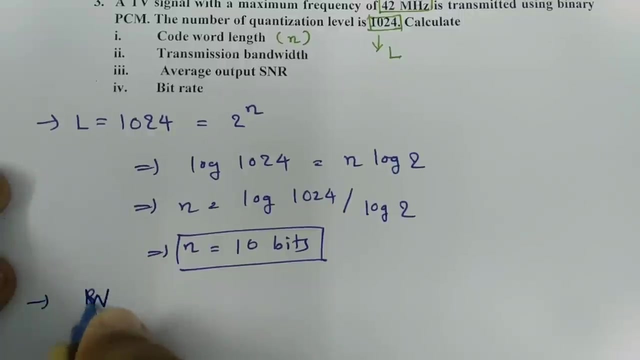 Here, per sample, we are delivered to take 10 bits And bandwidth of signal that is 42 megahertz. So here see bandwidth, That is 42 megahertz. Bandwidth of signal, let us represent it by W, that is 42 megahertz. 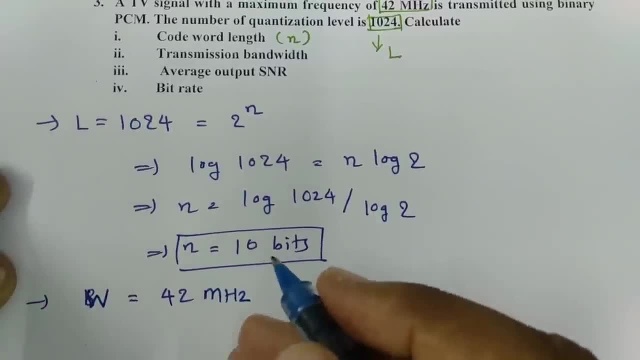 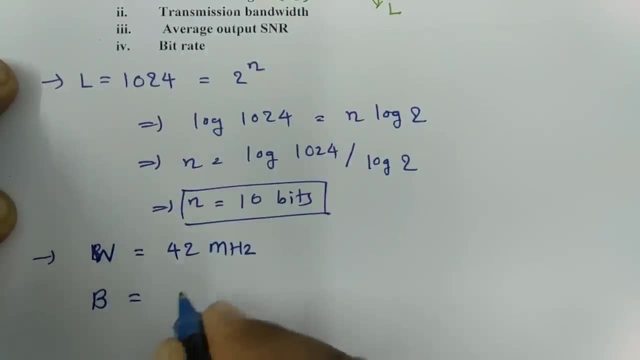 And per each sample we have 10 bits. So actual transmission bandwidth, Actual transmission bandwidth, that will be N times of bandwidth of signal, So it will be N into W. The reason is each sample requires 10 bits, So you will be having total transmission bandwidth, that is number of bits into W. 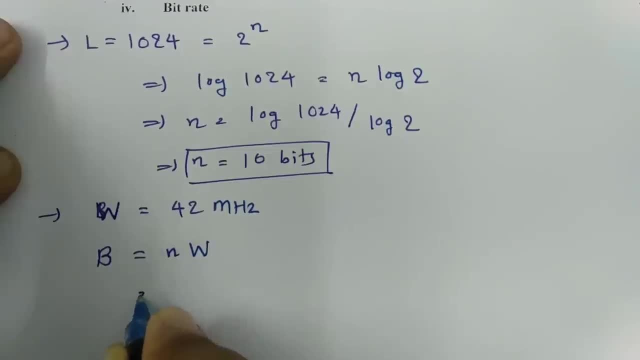 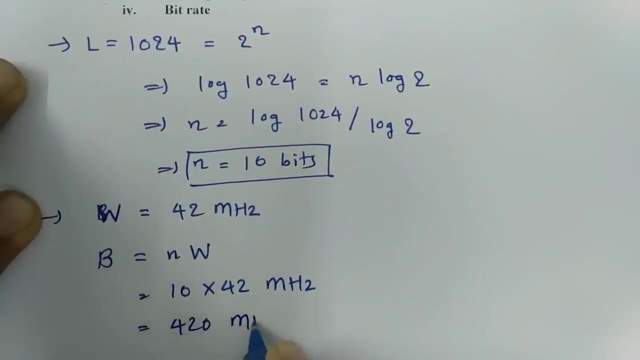 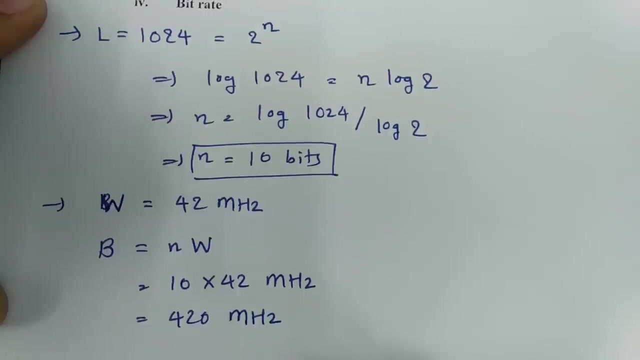 So at the end you will be getting: N is 10 and bandwidth is 42 megahertz. So this bandwidth, that will, be sorry, 42. So that will be 420 megahertz. So bandwidth required, that will transmission bandwidth, that will be 420 megahertz for this. 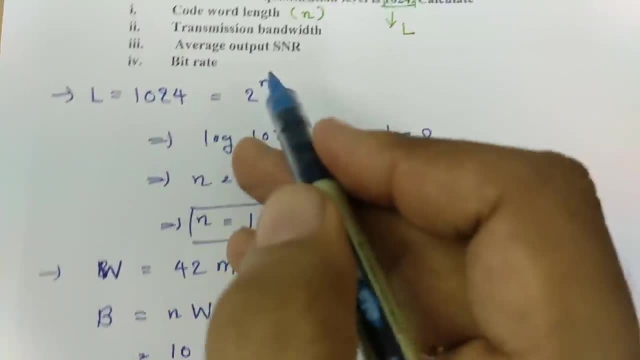 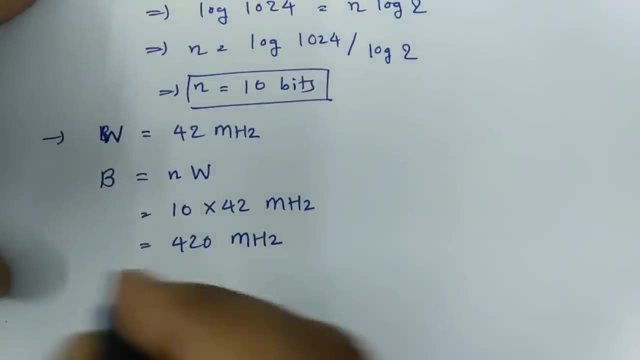 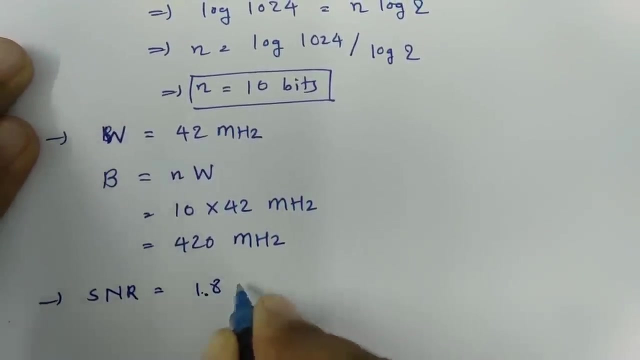 Now next question is to solve average output SNR. So average output SNR, as this signal is sinusoidal signal of TV signal, We can calculate SNR And that SNR that will be, as per this calculation, 1.8 plus 6N. 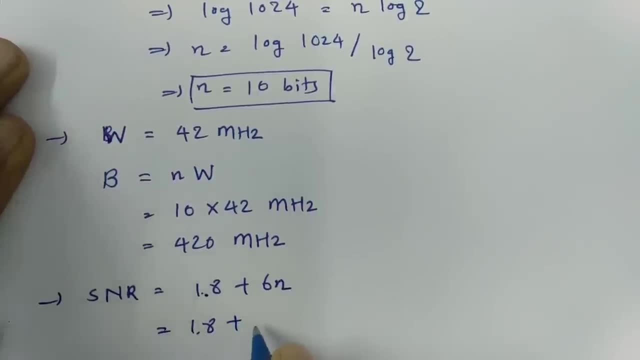 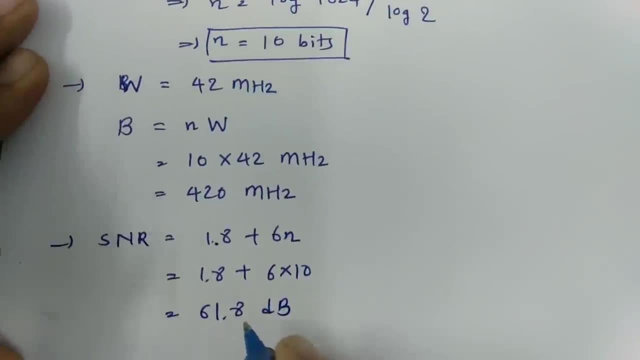 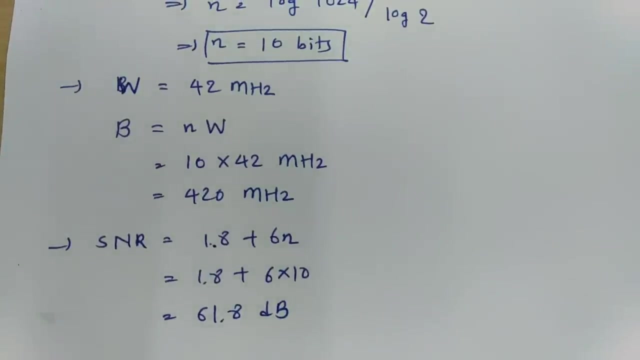 1.8 plus 6 into 10.. So 60 plus 1.8 that will be 61.8 dB. So 61.8 dB, that will be SNR of this signal. Now next question is: calculate bit rate. 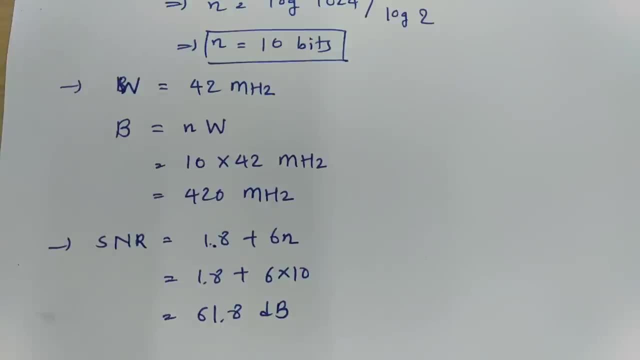 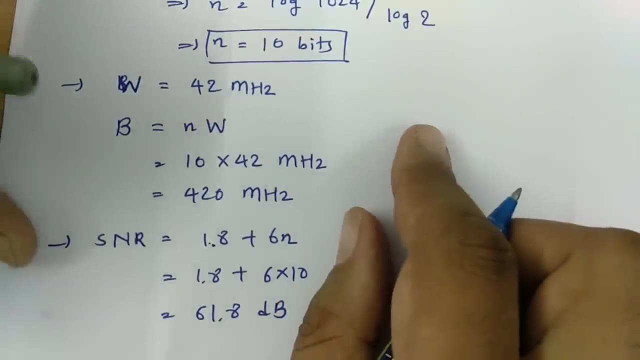 So what will be bit rate? Now see, bit rate is quite interesting. Now, before I exactly explain how to calculate bit rate, Let us try to understand what will be sampling rate. So sampling rate, that will be twice of this bandwidth. 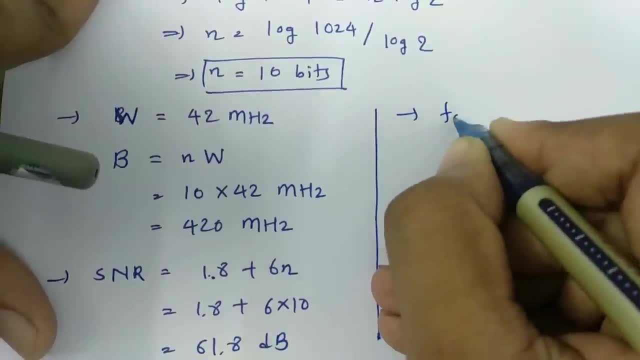 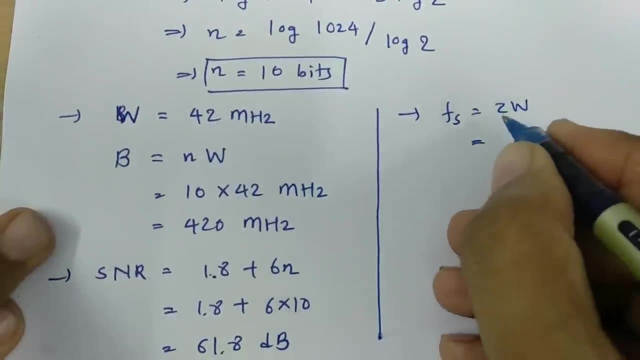 So I am just calculating it here. Sampling rate Fs, that will be twice of bandwidth. So that is what we have already derived based on sampling. So sampling rate is twice of bandwidth. So 2 into bandwidth is 42 megahertz. 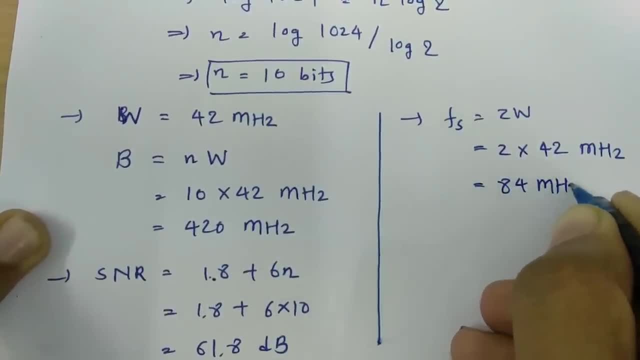 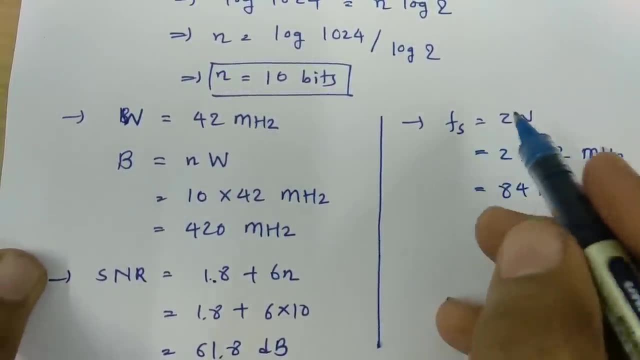 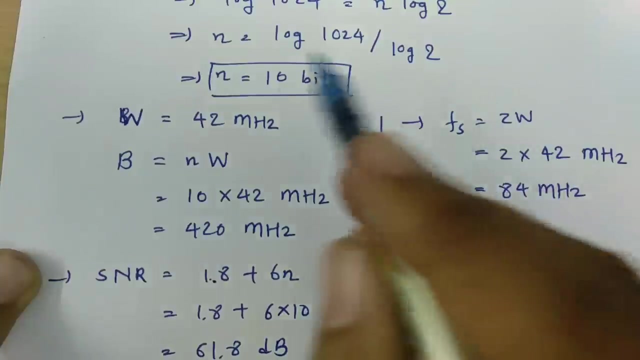 So you will be getting this will be 84. Now you just see sampling rate. that is 84 megahertz. So what will be bit rate? Now see bit rate. that will be actually number of bits per sample. means sampling rate into number of bits. 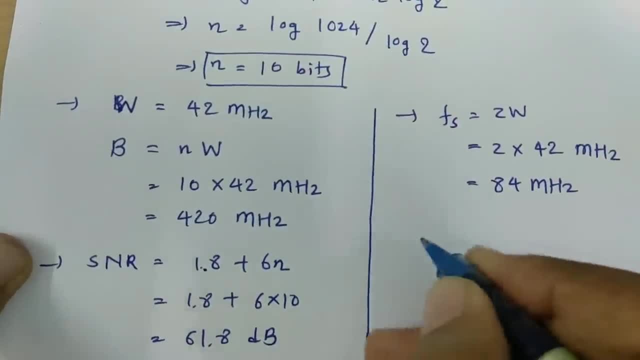 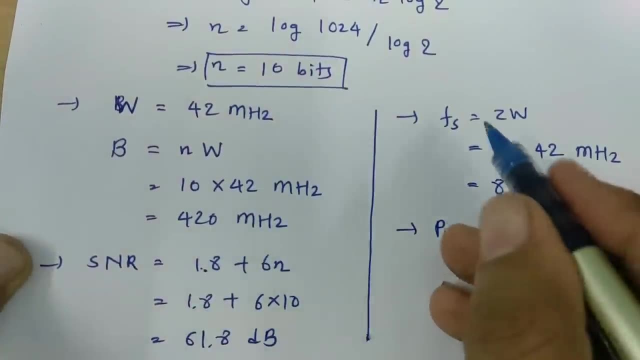 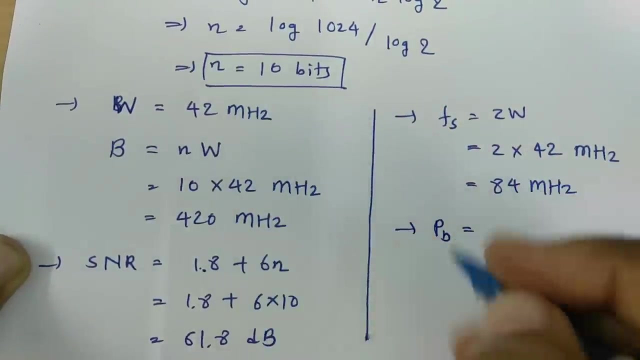 That is what bit rate. The reason is, if I say PB, that is bit rate, then per each sample it requires to have 10 bits. So at sampling rate At least, you will have to have Fs into N. that will be the bandwidth bit rate of that. 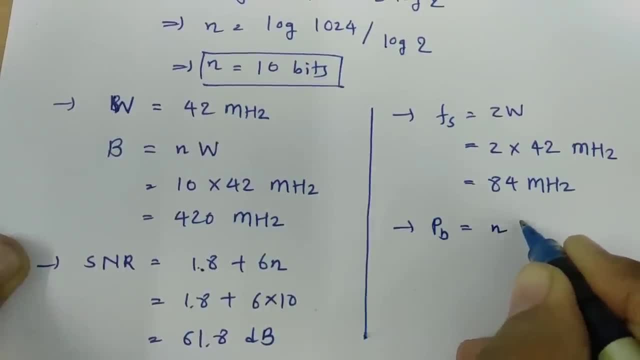 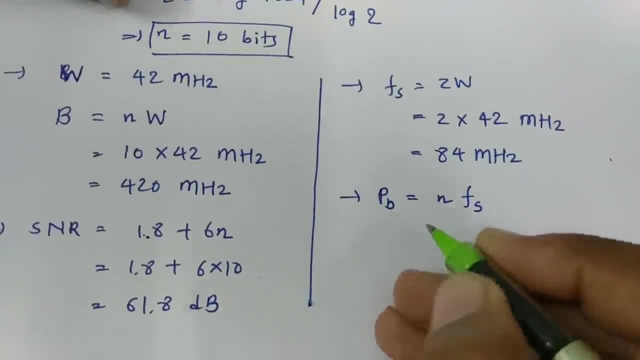 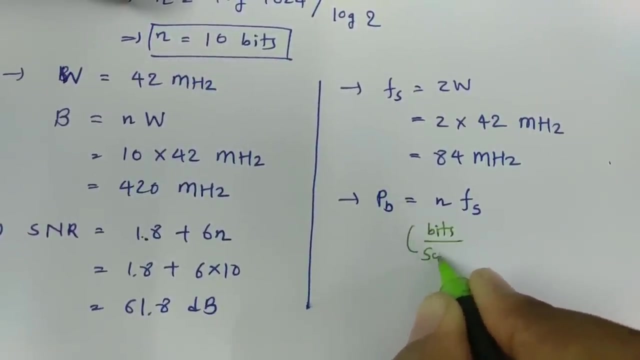 So you will be getting this will be N times of sampling rate. Now here one should understand how this is happening, Why this is bit rate. So see, N is what number of bits per sample. N is what number of bits per sample. 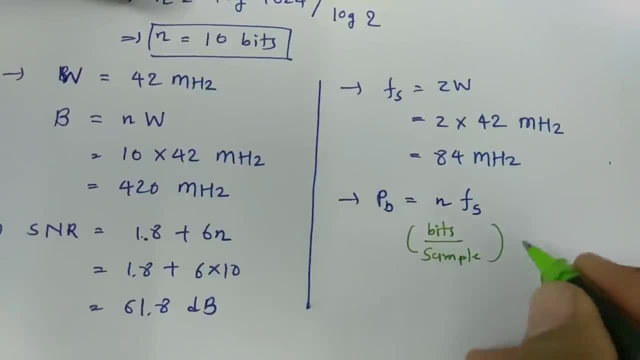 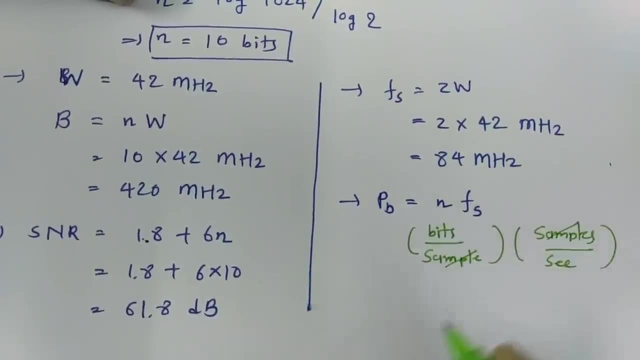 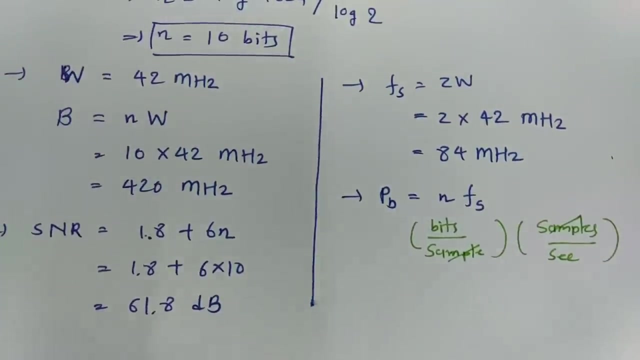 And Fs is what rate of samples means it will be samples per second. So here sample samples will get cancelled And this will be actually bits per second. it is what bit rate? So when you calculate this, you will be getting bits per second. it means this is what bit rate. 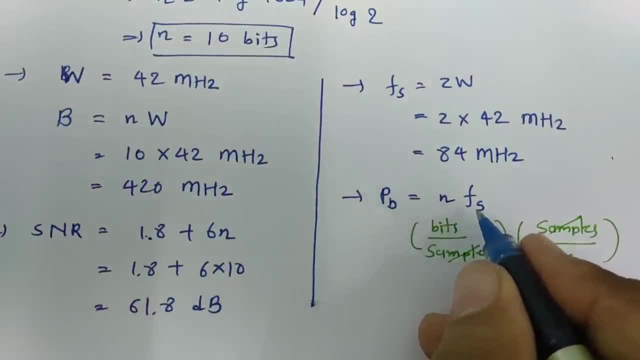 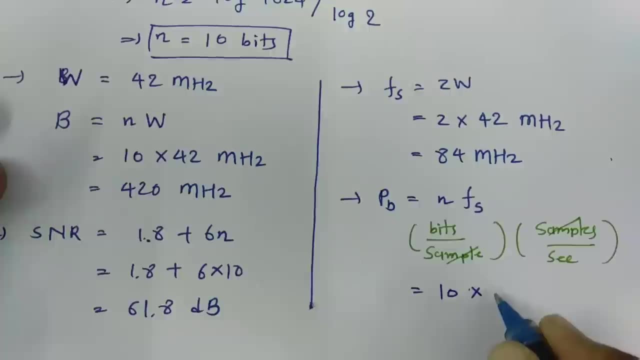 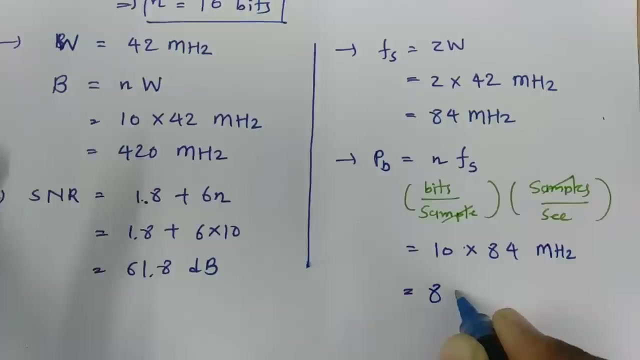 So bit rate is actually number of bits into sampling frequency And you will be getting this as per 10 into sampling frequency that is 84 MHz. So you will be getting this is 840 Mbps. The reason is: now you will be getting that in terms of bits per second. 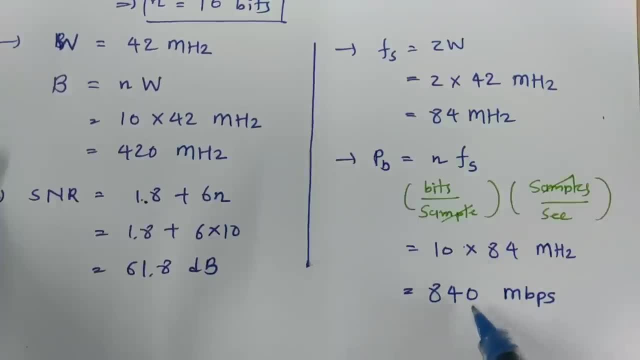 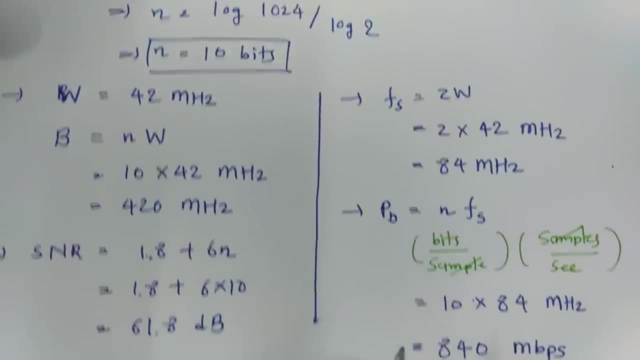 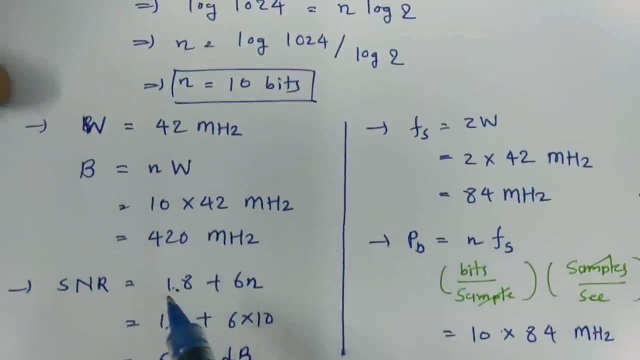 So it is what? MHz So you will be getting, this will be Mbps. So here again one should look at in brief like: see, if sinusoidal signal is there, then one can use SNR formula by this And they can directly calculate all those data as per this calculation which I have done. 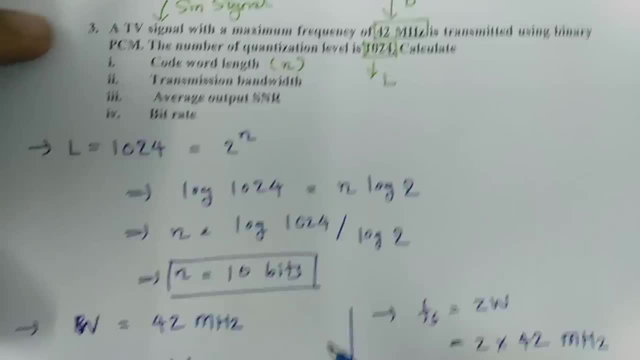 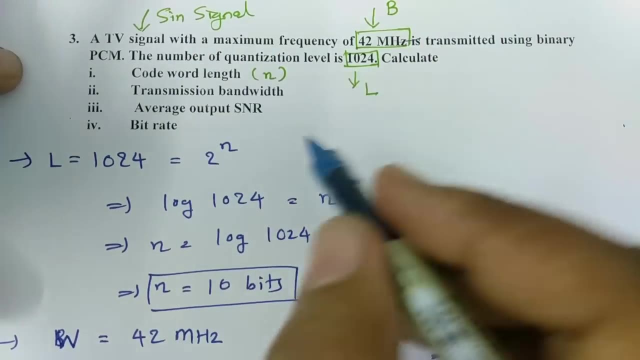 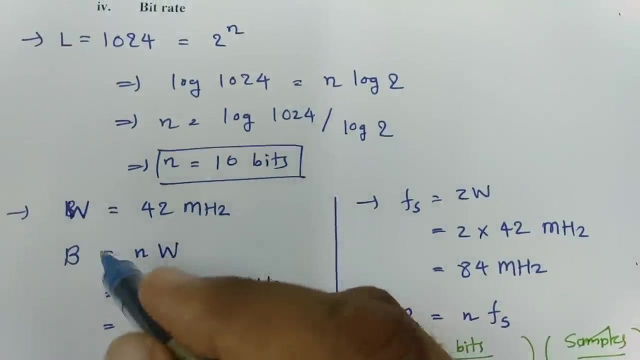 L is what 2 to the power N. from that you can calculate number of bits. Bandwidth of signal means highest frequency of that input signal And here levels are given. So from that bits will be calculated. So bandwidth of signal we can have bandwidth of sampling. 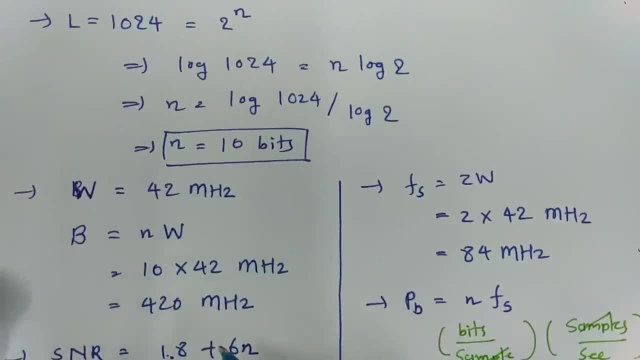 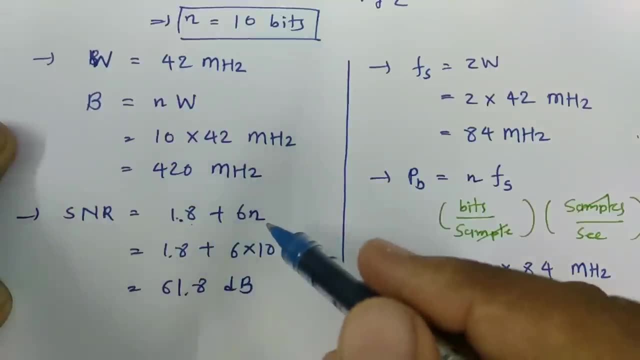 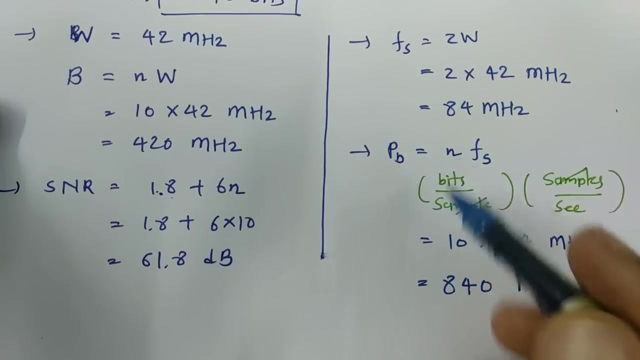 And bandwidth of sampling is what? bandwidth into number of bits per second. So that will be bandwidth, transmission bandwidth and SNR is 1.8 into 1.8 plus 6 N in terms of dB And when you calculate data rate, bit rate in digital, then it will be number of bits into sampling rate.